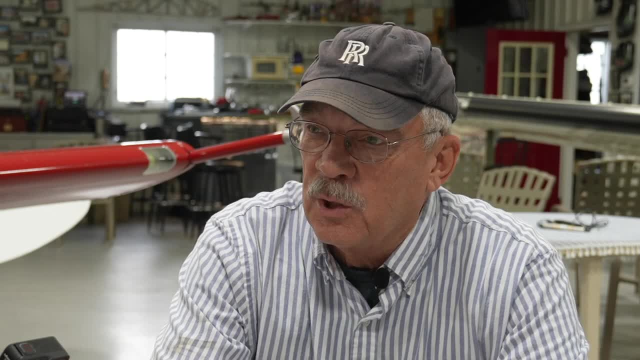 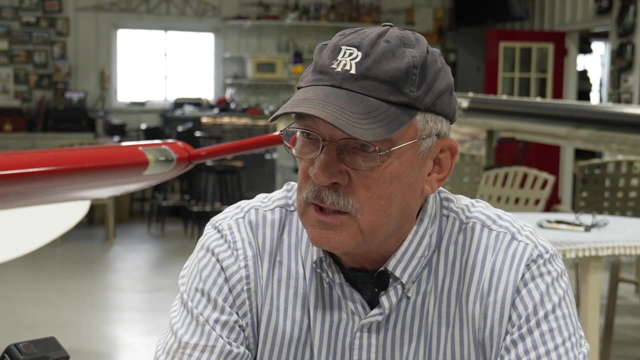 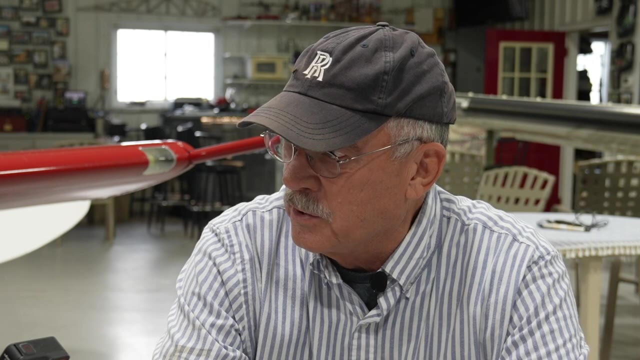 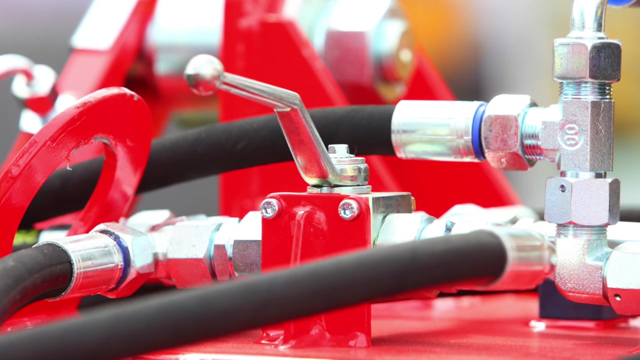 concept of how their electrical system works, And so, over the years, I've figured out a way to explain the electrical system that pilots seem to be able to better understand, And that is by comparing the electrical system to a hydraulic system. It's a lot easier to visualize oil moving in a pipe, Yes, And whether it's a pump or an actuator. 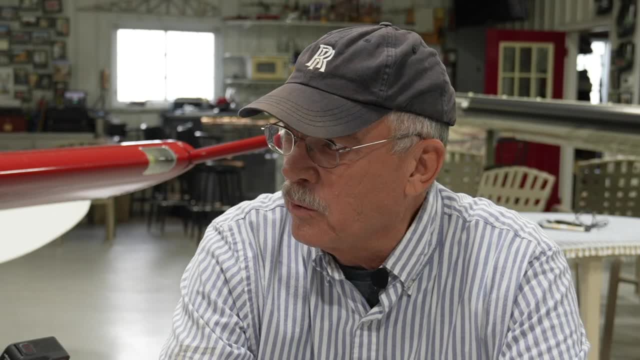 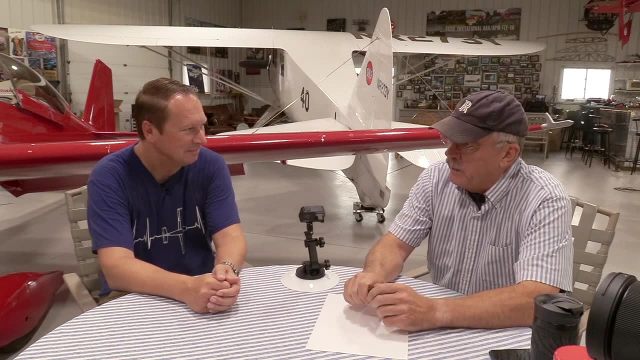 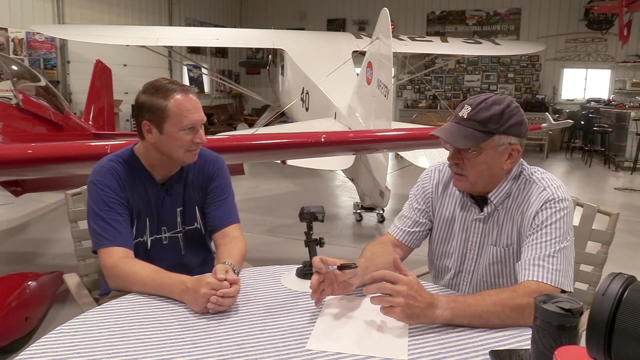 But in reality, the electrical system and the hydraulic system operate almost identically, And so what I do is start with the. where's the electrical system? Where does the electricity come from? And, as an engineer, how would you answer that question? 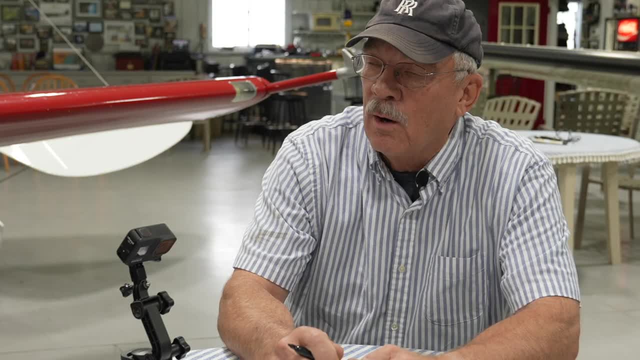 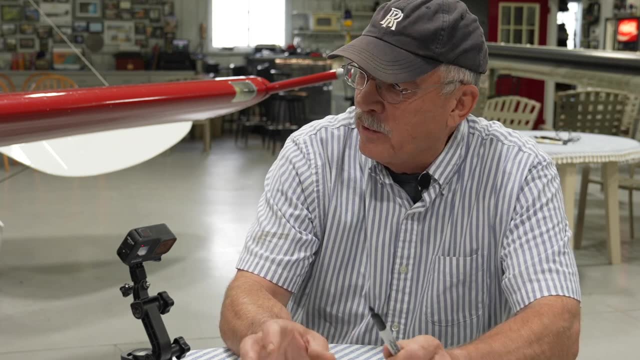 It's a power source like a battery or the alternator. Okay, So the alternator and the battery is where it comes from, But I was being more basic than that. Where does the fluid come from? In the hydraulic system, it comes out of a reservoir. 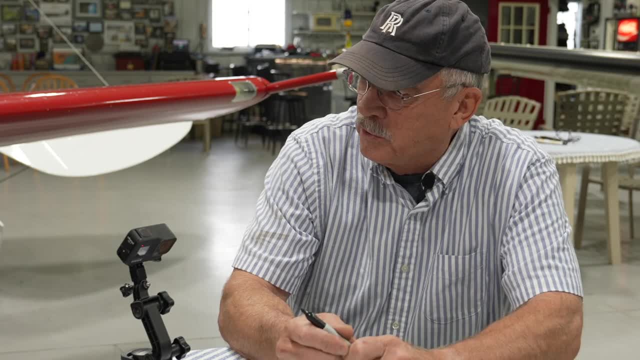 Where does the motive flow in an electrical system come from? It's the electrons in the conductor, That's right. And they come out of- I've heard it described as the e-flow- And that's where the electrons come from. And that's where the electrons come from And that's where the 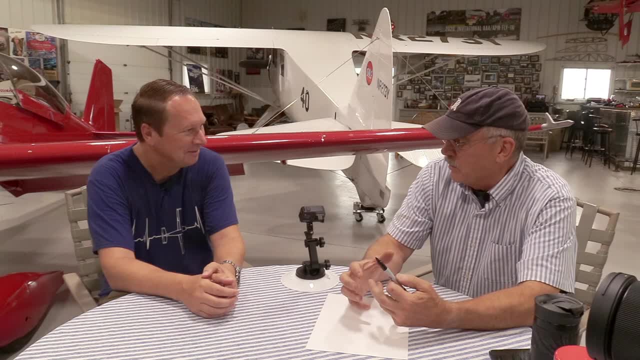 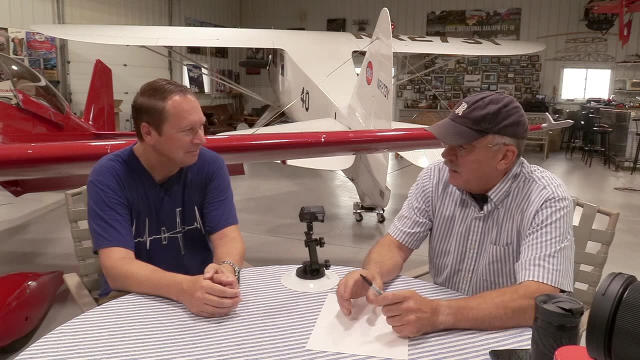 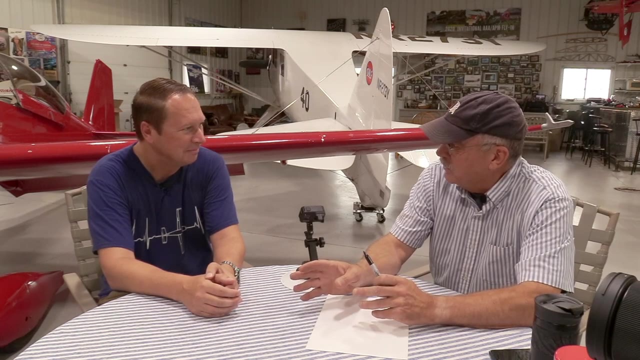 Yeah, That's right, We pull them out of the atmosphere in some manner or form. But our motive flow in a hydraulic system is oil And our motive flow in an electrical system are electrons. And Boeing builds electric airplanes. And back in World War II North American built hydraulic airplanes. And I would 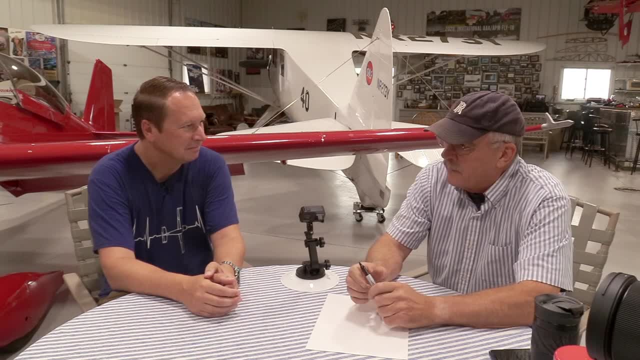 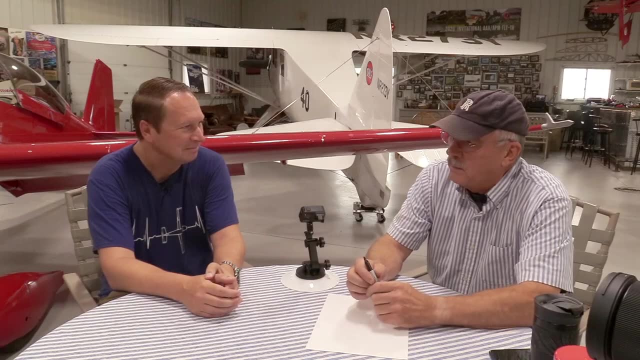 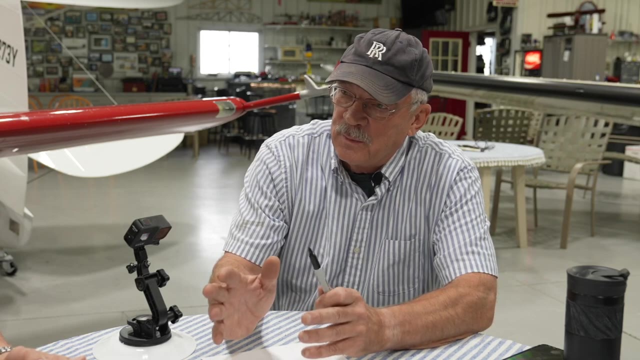 argue that one of the drivers behind an electric airplane over a hydraulic airplane is that you never run out of hydrogen Hydraulic fluid Because you can always make more. But so, understanding that the motive flow in the hydraulic system is oil and the comparable in the electrical system is electrons, then we go to just 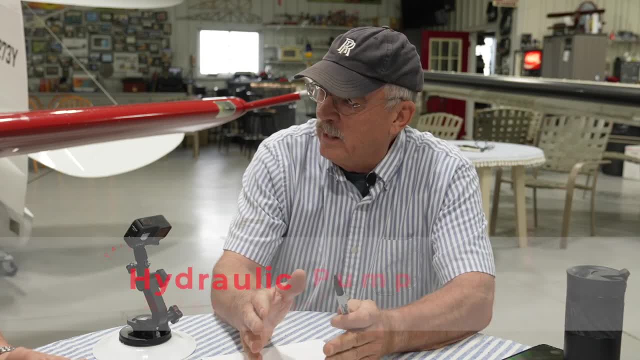 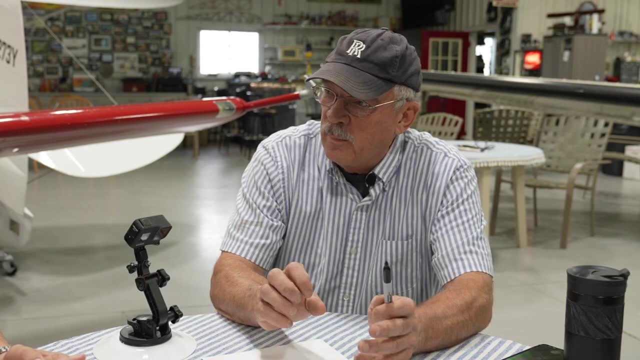 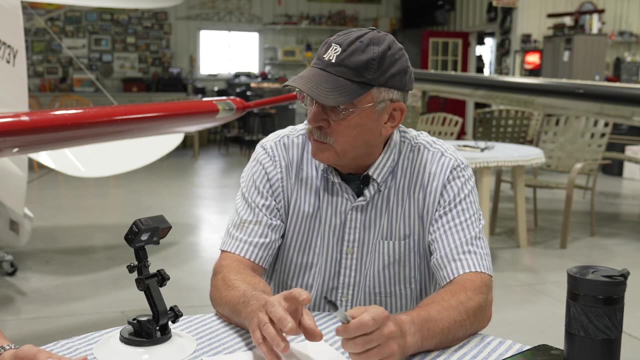 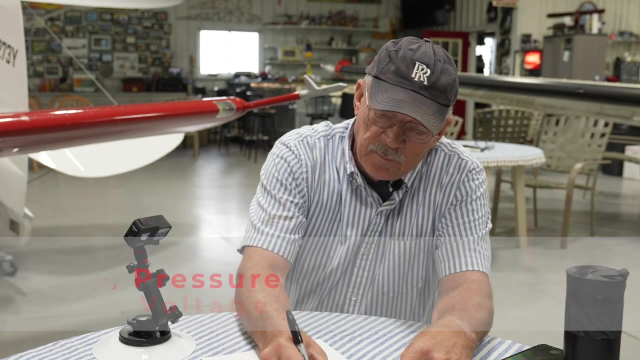 exactly what you said. Our hydraulic pump is a alternator or generator, right, Right. And so we take oil or electrons and we pressurize them. Okay, So we all understand the concept of pressure. Well, in the electrical system, pressure is volts, Okay. So we got volts equals pressure, Okay, And so now we move. 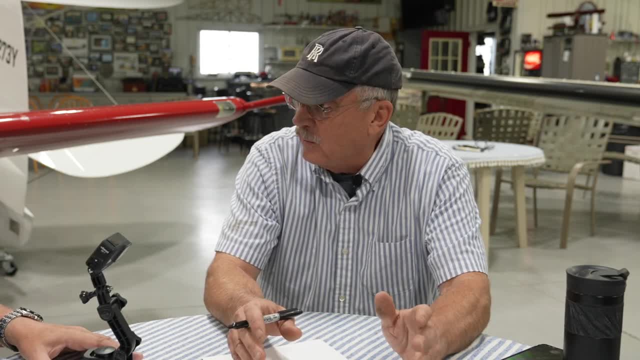 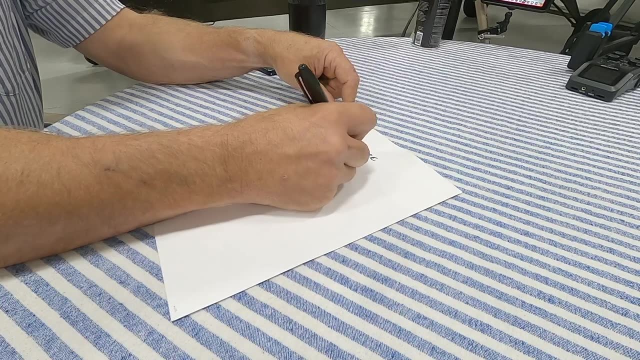 oil in the hydraulic system at a certain gallons per minute. We call that flow right Right. So in an electrical system we would call or in a hydraulic system we would call that gallons per minute. In the electrical system we call that. 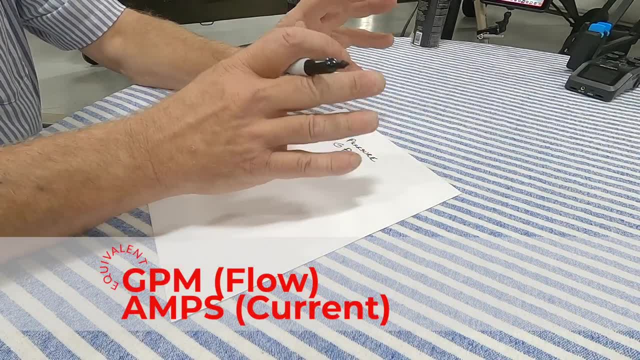 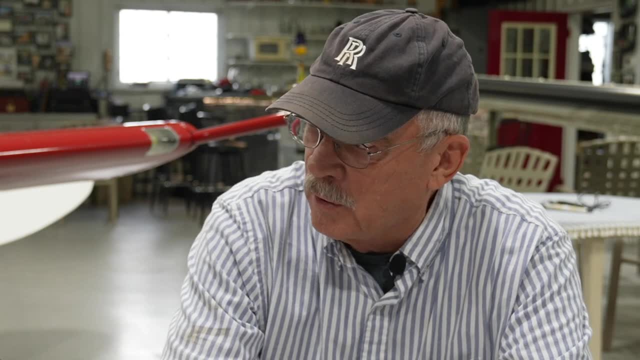 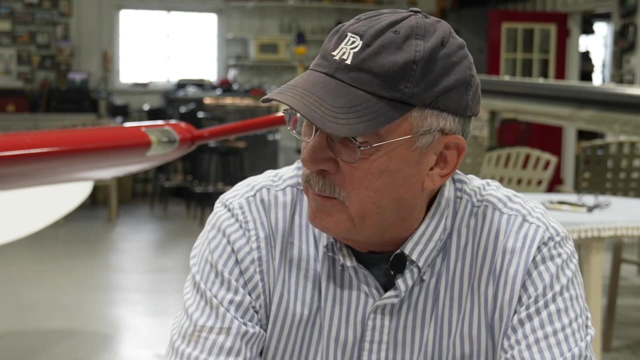 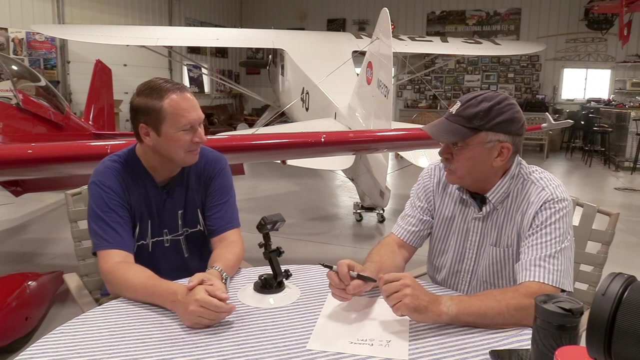 amps. Yes, Okay. So now that we understand that the generator or the hydraulic pump make pressure or voltage and the amount of oil they move or electrons they move is gallons per minute or amperage- Current, Current, That's right- Which we measure in amperage, That's correct. 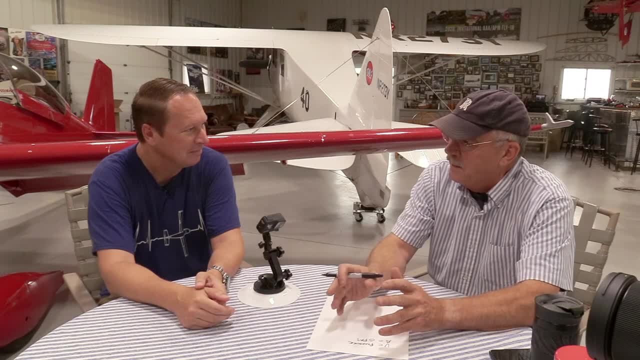 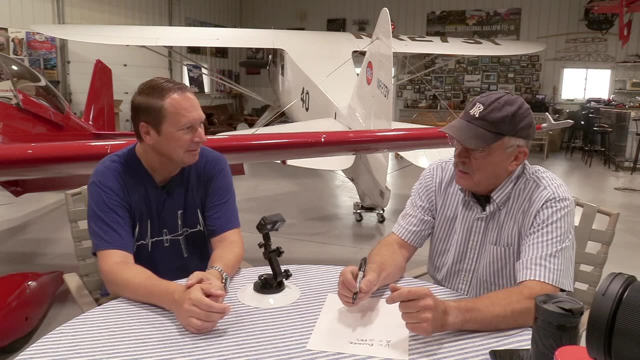 Current is measured in amperage. I never thought of it that way. Current, like the metric current in a river, is how fast the water flows exactly. that's an easy way to remember that I'd never thought of that. okay, so after the oil comes out of our 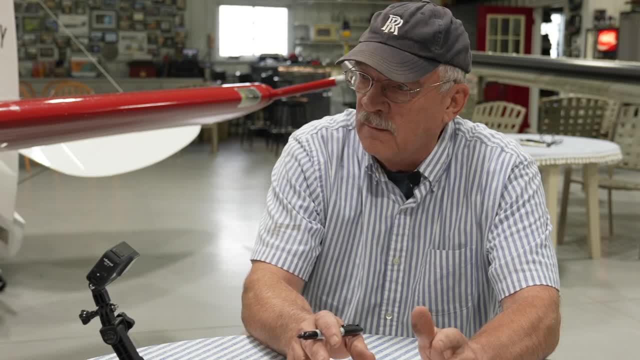 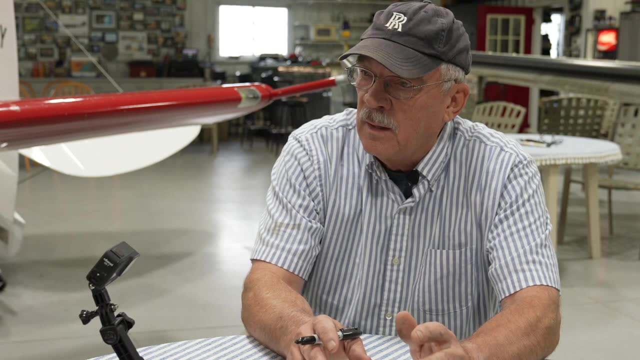 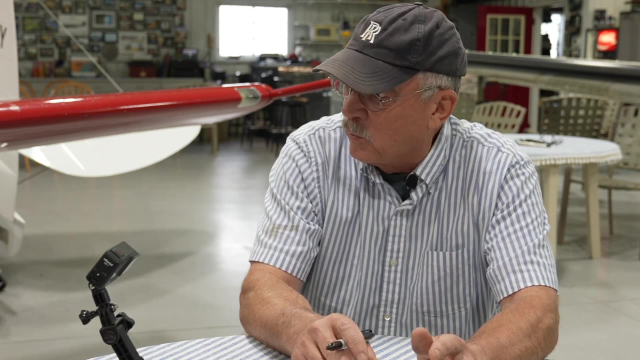 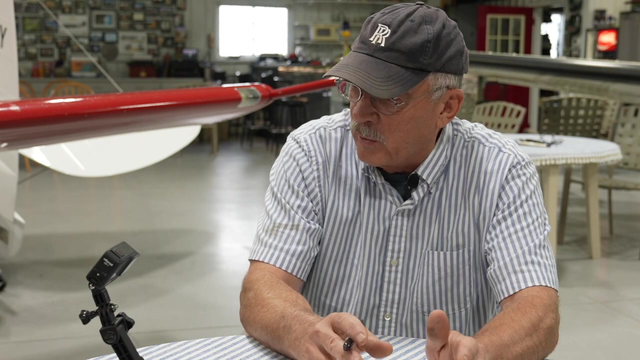 hydraulic pump. usually we have some sort of device that regulates the pressure: pressure relief valve, a- it might be a return, you know- unloader valve that returns oil back to the reservoir at low pressure, but so we would call that. in a hydraulic system we would call that a pressure regulator, and in the electrical 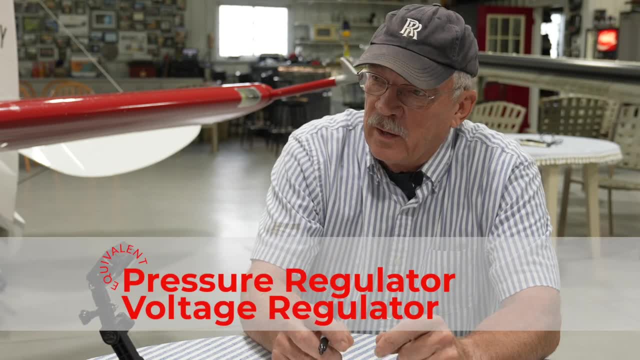 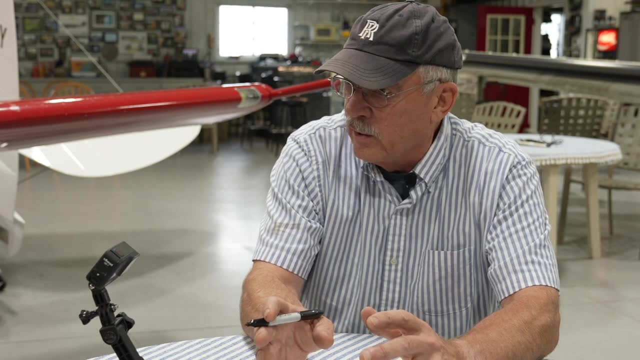 system, we would call it a voltage regulator. sure, now, very often in the hydraulics system, we have two regulating methods. one would be the normal system, which would be, like I said, an unloader valve or something that dumps low pressure fluid back to the reservoir and then 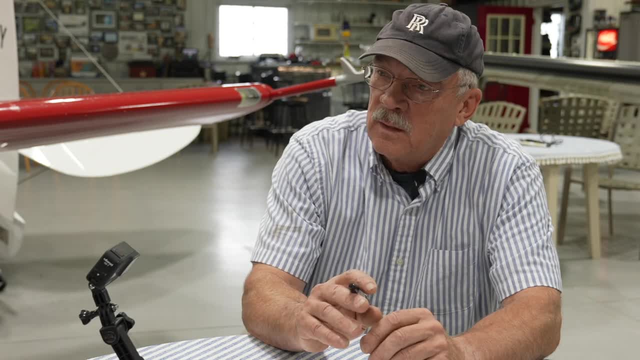 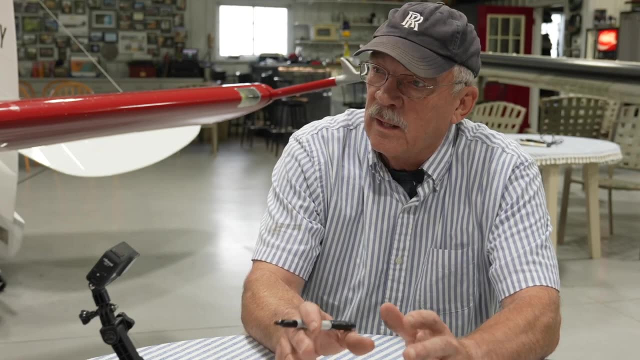 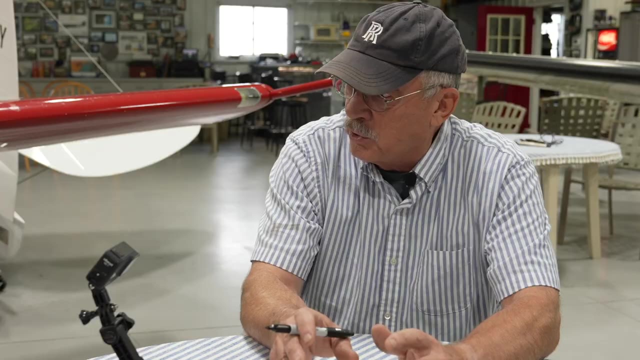 we have кая, a higher setting that depressurizes the system in case of an emergency, and that'd be an emergency relief or overpressure relief valve. So in the electrical system the equivalent is obviously the voltage regulator, and then in some cases we have overvoltage protection. 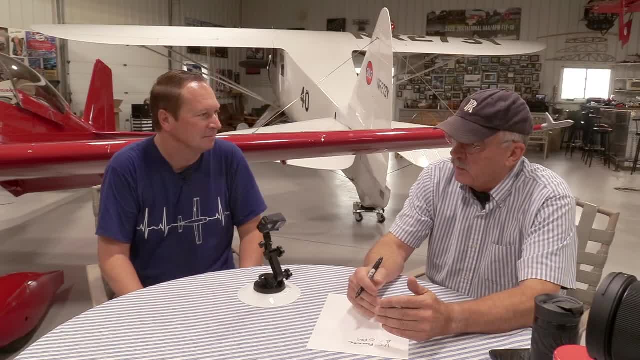 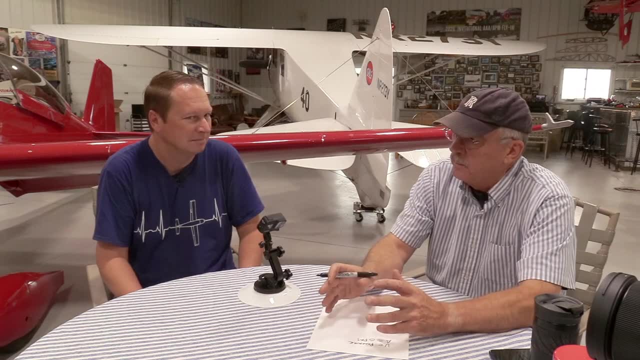 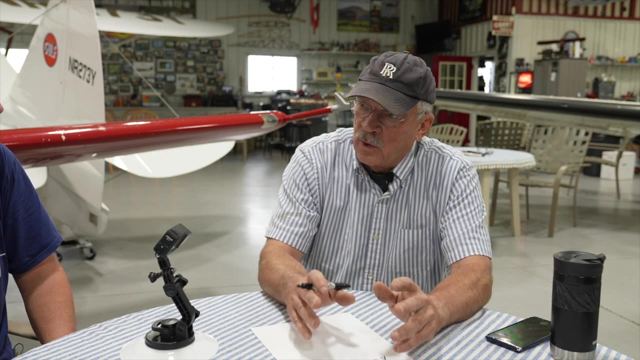 After the pressure regulating system, in either or the voltage regulating system, our energy has to go somewhere to be stored. People understand this pretty well: in electricity. In electricity we store our energy in a battery, In a hydraulic system we store it in an accumulator, which is typically either a piston or a diaphragm. 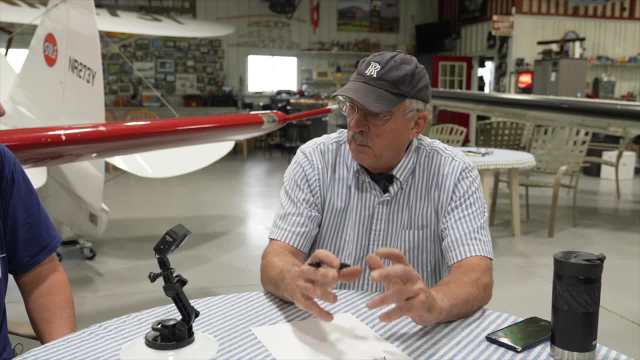 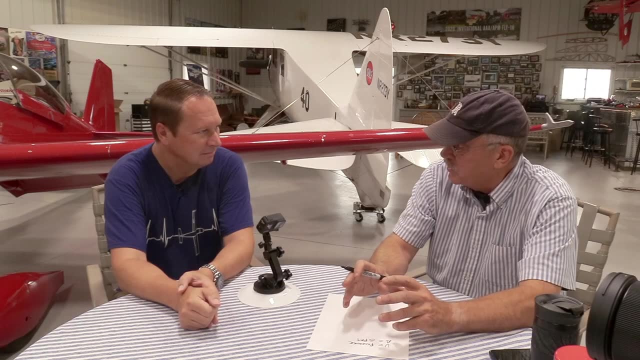 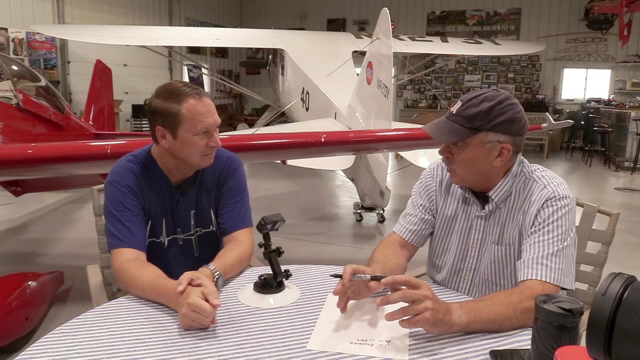 with compressed gas or a spring on one side and motive flow oil on the other side, And that does a lot of things: takes the surges out of the hydraulic system and it allows for the pump not to have to cut in so often. 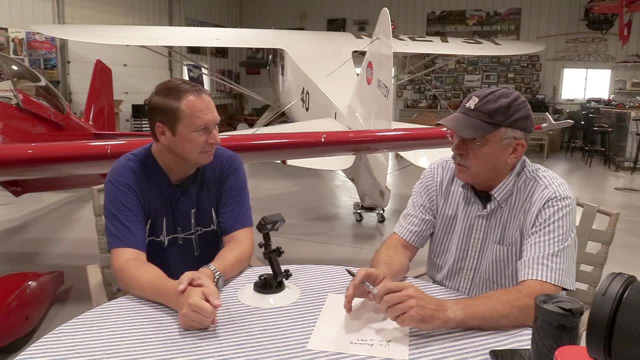 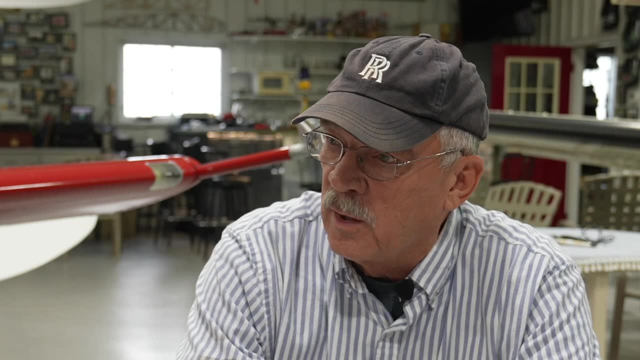 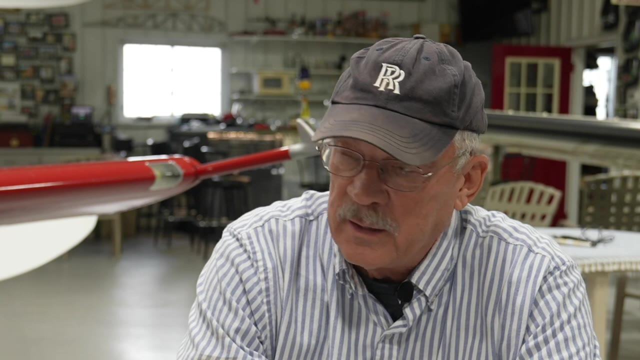 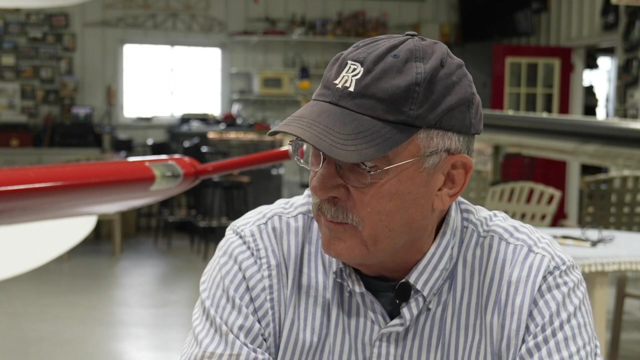 And in the case of the failure of our pump, the accumulator can provide us with one or two applications of brakes, might have enough capacity to put the gear down, And the battery does exactly the same thing. The battery actually is probably a better accumulator because it has more capacity than. 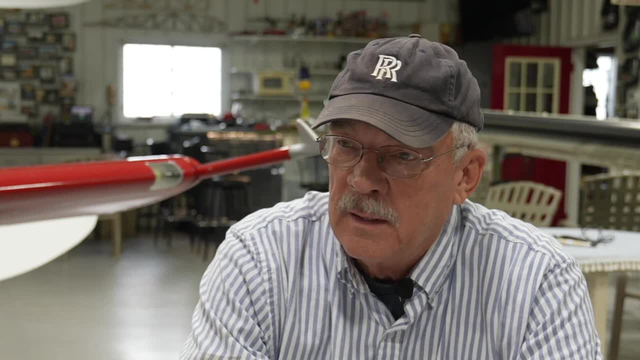 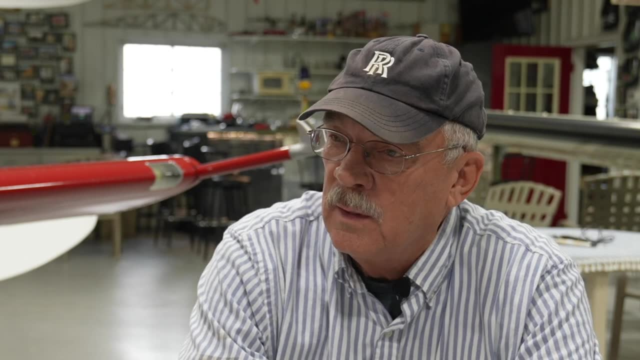 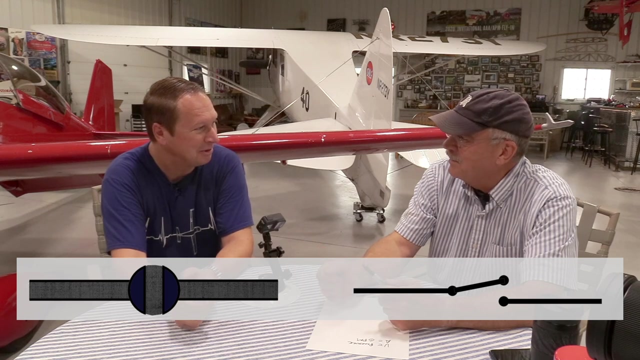 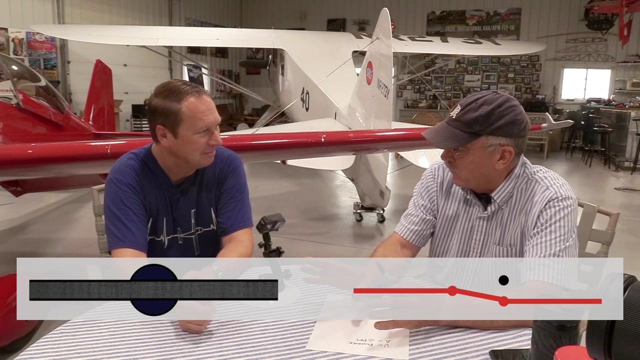 a hydraulic accumulator, but it serves the same function. Okay, Then we come to controlling the flow and utilizing it. The electrical equivalent of a hydraulic valve would be a switch, That's right. Electric switch: That's right. It diverts or interrupts or connects the motive flow to whatever it is that we want to have. 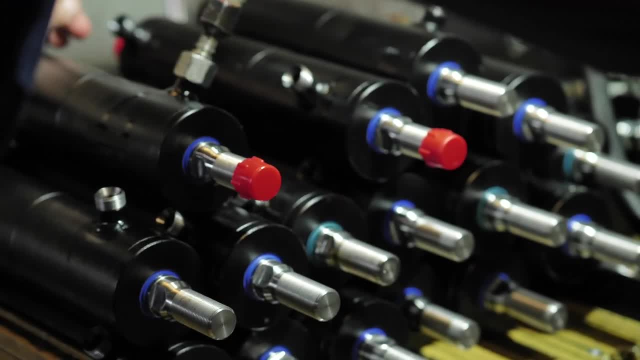 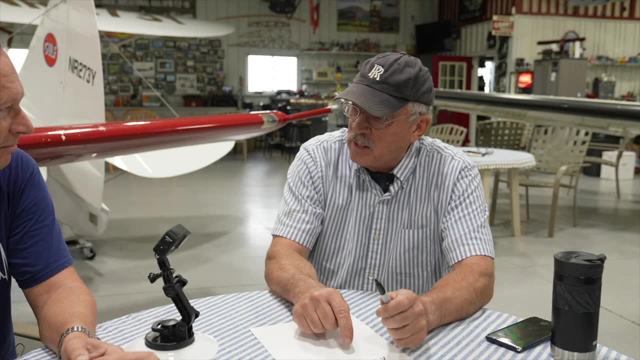 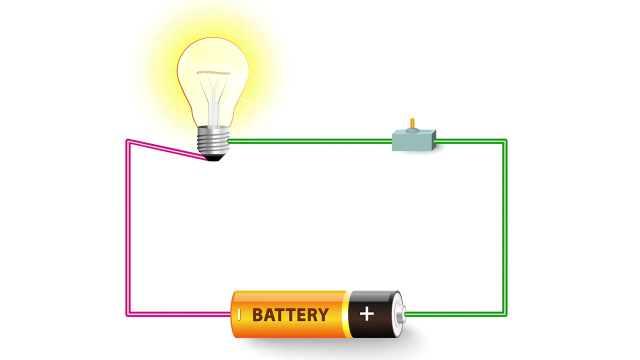 that does work, Then we run the hydraulic fluid. If we open the valve, the hydraulic fluid either runs to a cylinder or a motor, where it creates work. In the case of electricity, the motive flow electrons either go to a servo, a motor, a. 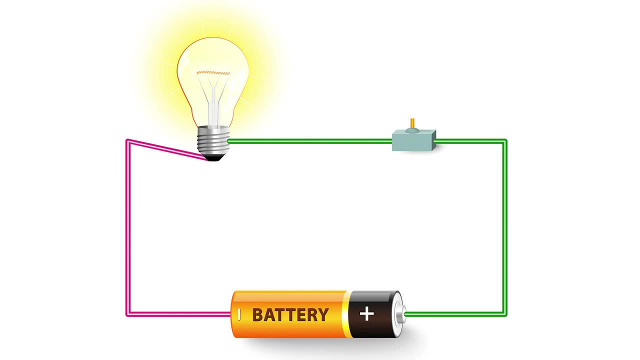 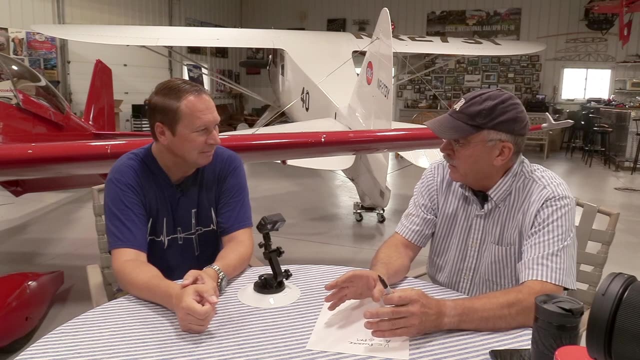 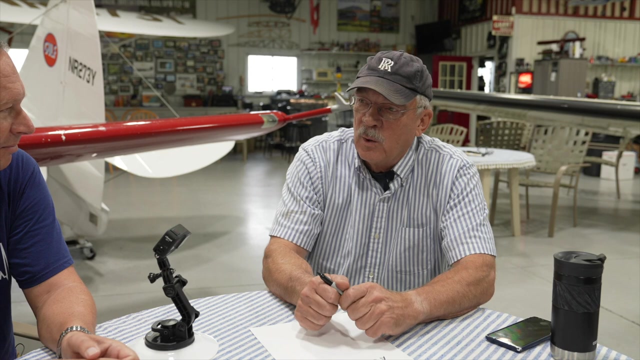 light bulb, whatever, and they create work. If we think about electricity in the terms of hydraulics, it becomes very simple and I think pilots can understand it. It's great to sit here at the table and talk about how the system works, but when it really 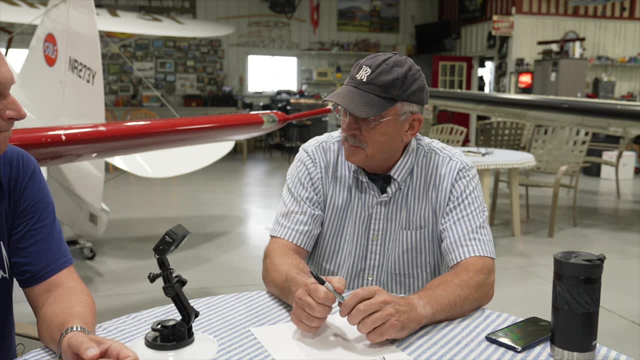 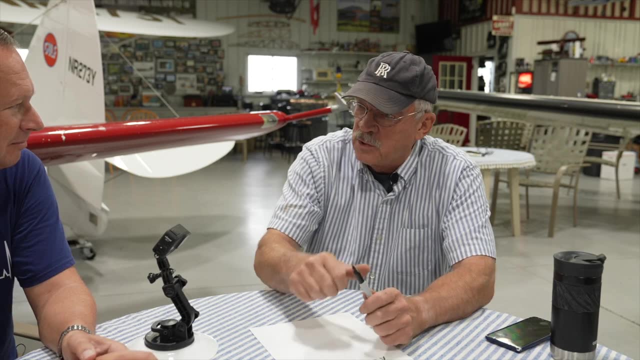 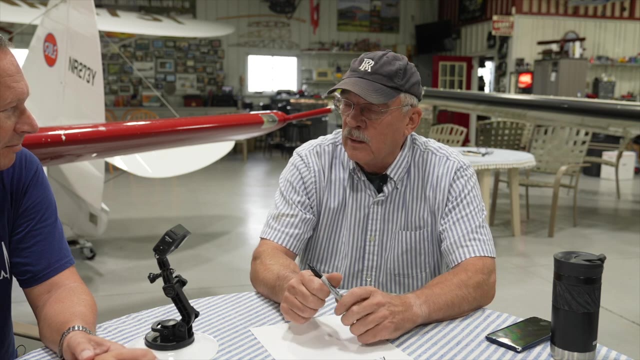 becomes important. That's when something goes wrong, when we have a problem. One of the questions I would ask on a type rating, where the level of knowledge is expected to be higher, is: if we look down, we're flying along in flight and we look down in a single. 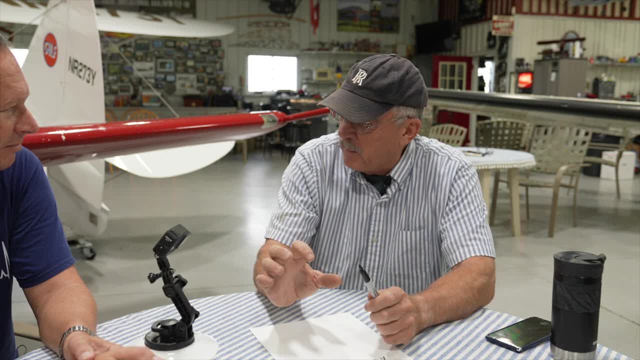 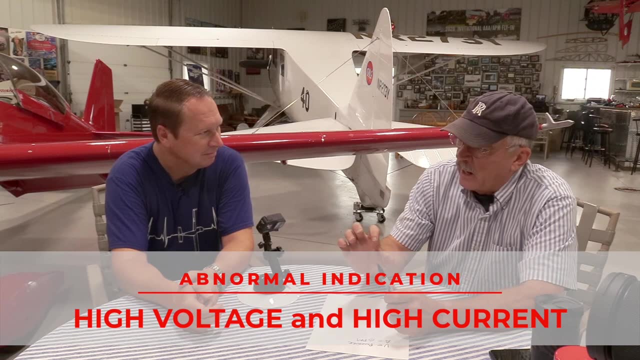 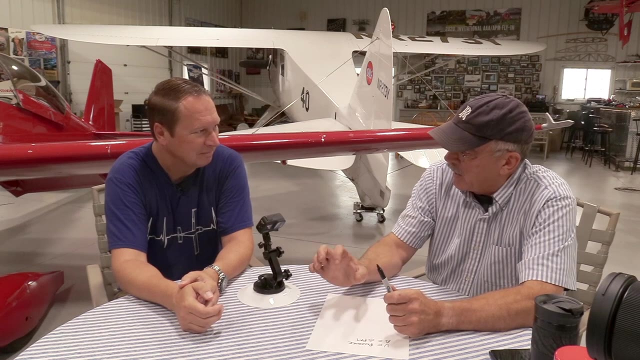 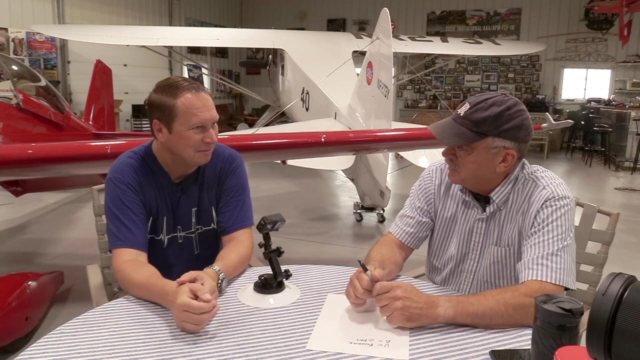 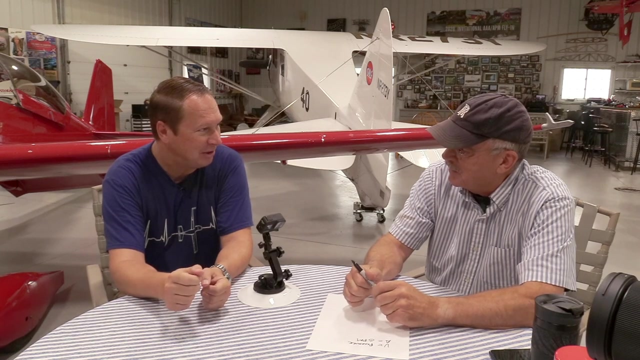 engine airplane at the volt amp meter and we see that the airplane has high volts and high amps. So that is the equivalent of high pressure and high flow. What could cause that? Well, if I look at the analogy with the fluid system, there's too much pressure, that is. 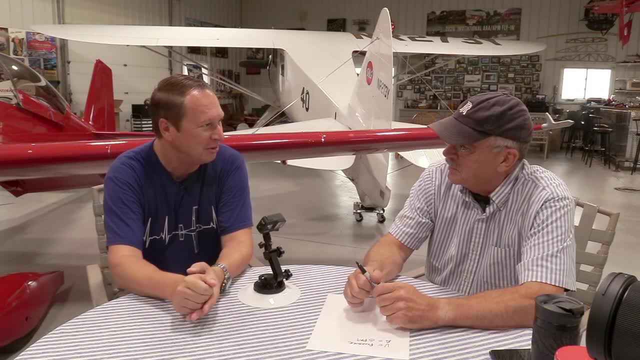 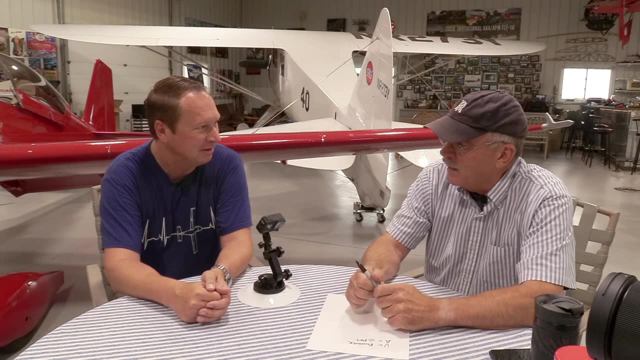 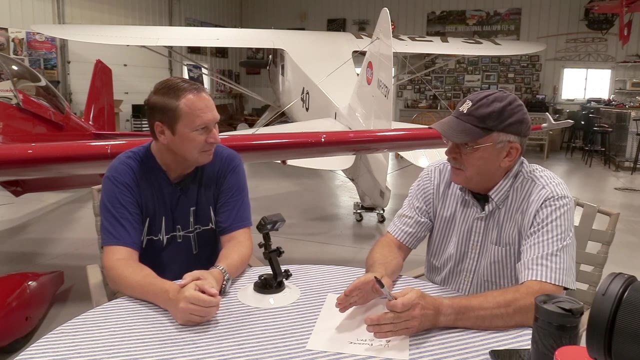 not stopped by anything, so it results in more flow than we normally see. So in the electrical system I would assume my voltage regulation, The voltage regulator, is defective. That is exactly correct. Putting out too much pressure on the whole system, That's right, because if you have too much pressure you're failing to regulate. That's really the only thing that can cause too much pressure. right is a failure to regulate. So we look immediately to the voltage regulator. Conversely, if we look down at our volts and amp meter and we see that we have high flow, 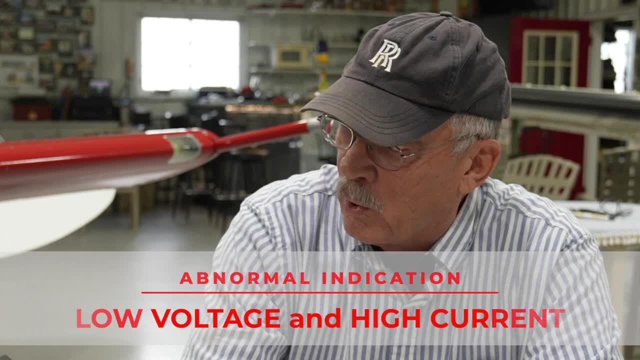 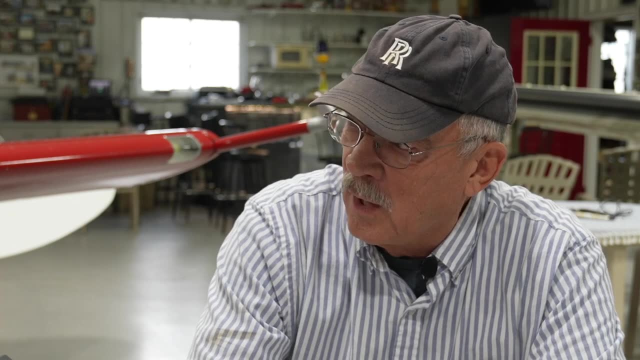 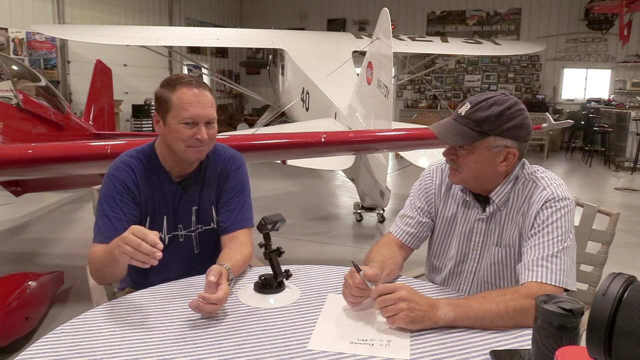 high current, High amperage and low pressure. going back to the hydraulic analogy, what would we expect to find in a hydraulic system? So if low pressure creates high flow, then somehow I must not have the full circulation with the consumers working, maybe a short circuit. 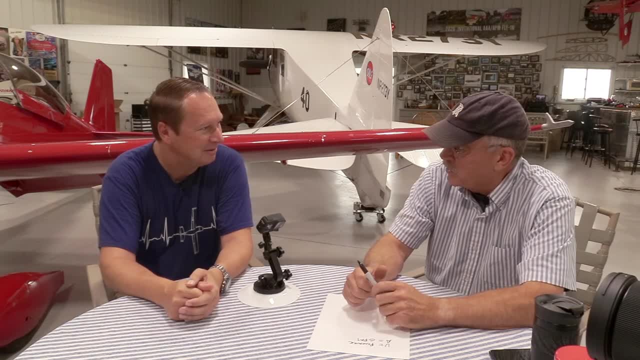 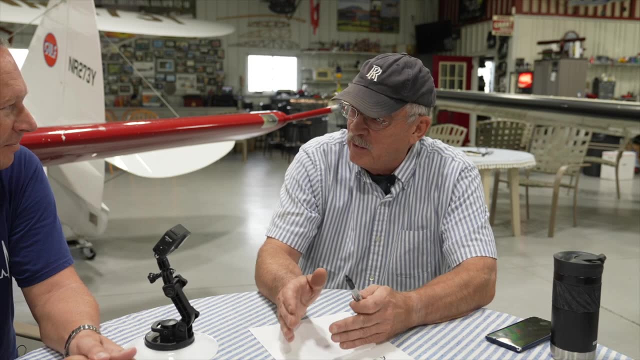 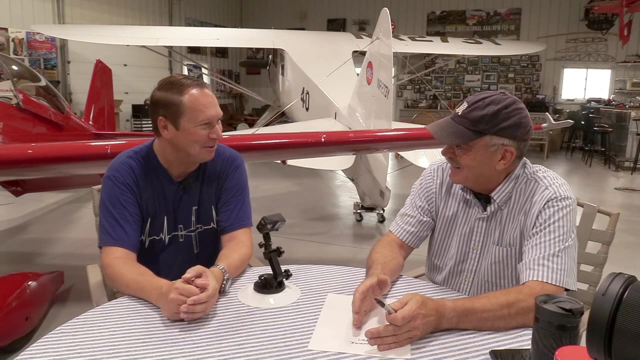 Well, or in a hydraulic system. A leak, A leak, A leak, And so the electrical equivalent of a leak in a hydraulic system is a short circuit. The good news in a hydraulic system is you quickly run out of fluid. If you call that good news. 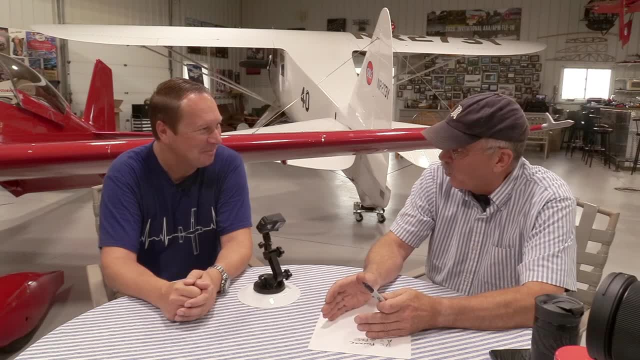 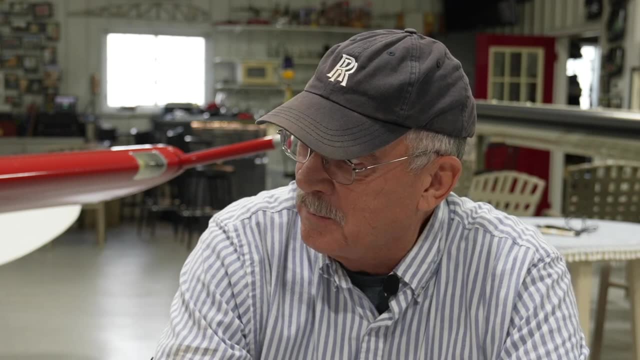 Yeah, The problem in an electrical system is we continue to make more fluid, right, And so when this fluid electrons exit the system, when they're lost, what happens? Well, I'm not sure, but it heats up. It heats. 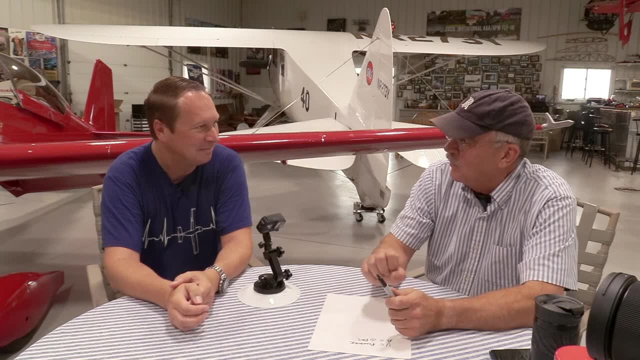 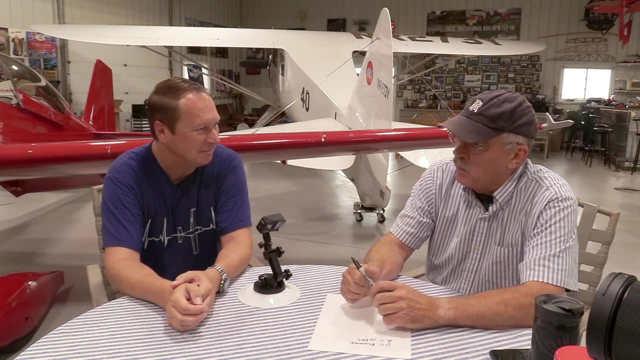 Yeah, So if we have a continuous supply, we're never going to run out of fluid electrons, And so the heat just continues to increase. So in the case of a hydraulic system, if we have a leak, there's probably nothing we can. 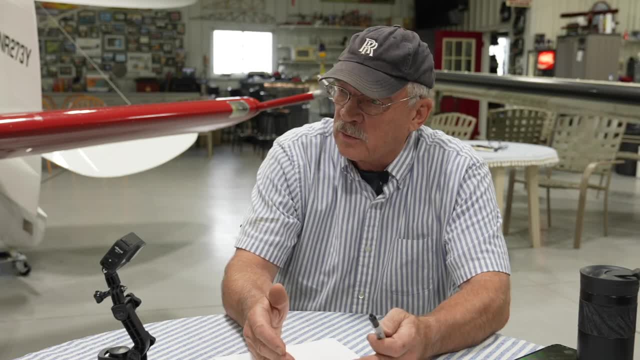 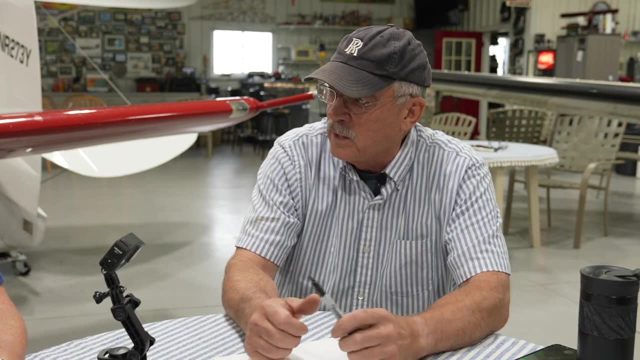 do about it And we run out of fluid and that's the end of the day. In an electrical system, if we have a leak or a short, it's going to continue to leak until we, as the pilot, take some action to eliminate the heat, eliminate the leak, which 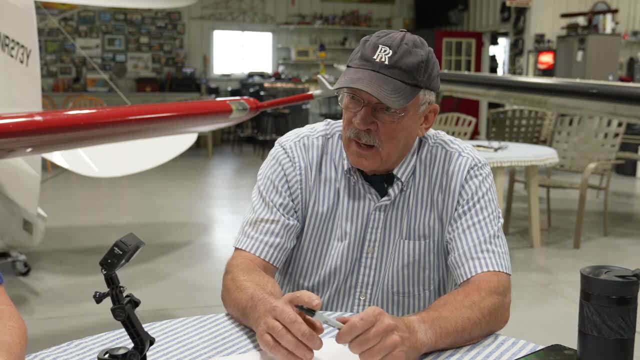 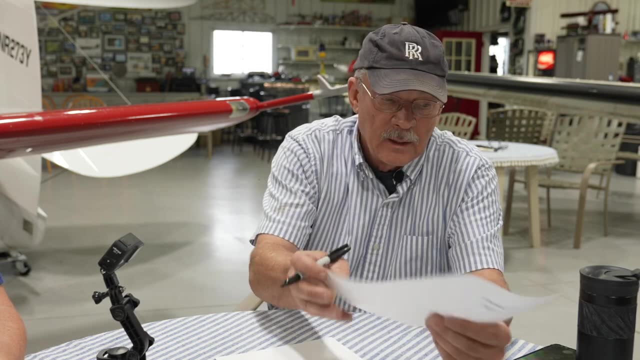 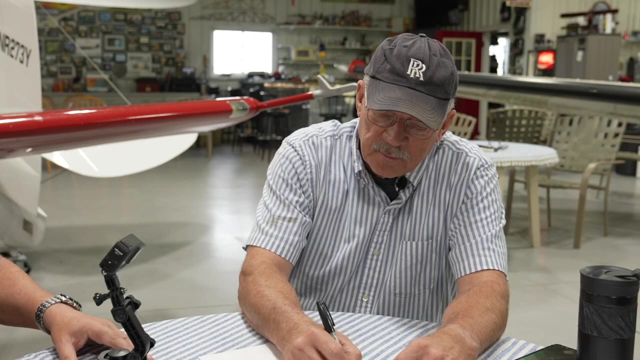 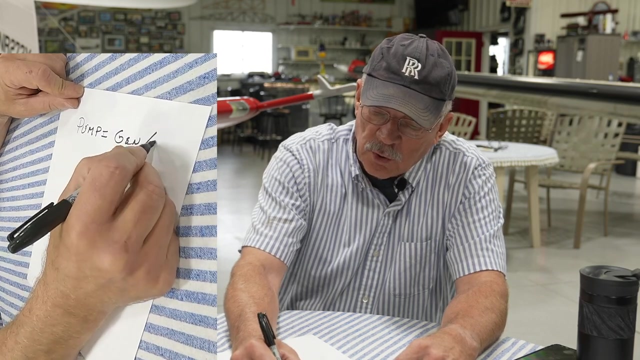 will eliminate the heat, And so I think, if we can equate the electrical system to the hydraulic system, pilots would have a lot better ability to understand that. So again, the pump equals the generator slash alternator. Okay, Mm-hmm. Yeah, Yeah, Yeah, Yeah, Yeah, Yeah. Cool. So if you have a higher voltage regulator, the regulator equals the voltage regulator, The high pressure relief equals the overvoltage protection, The accumulator where the motor flow goes Uh-huh. 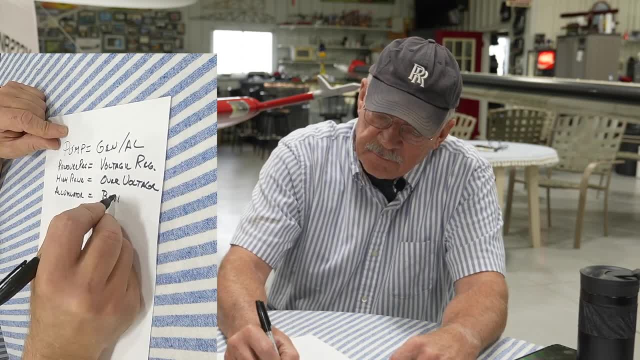 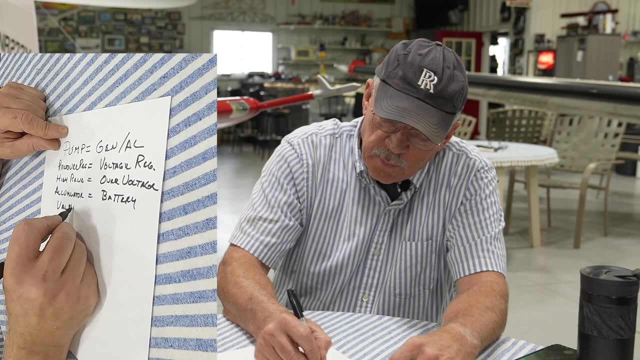 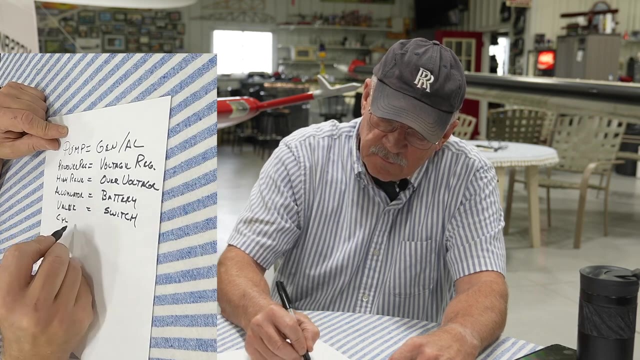 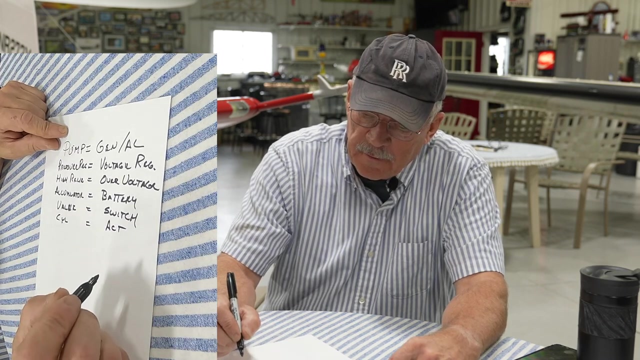 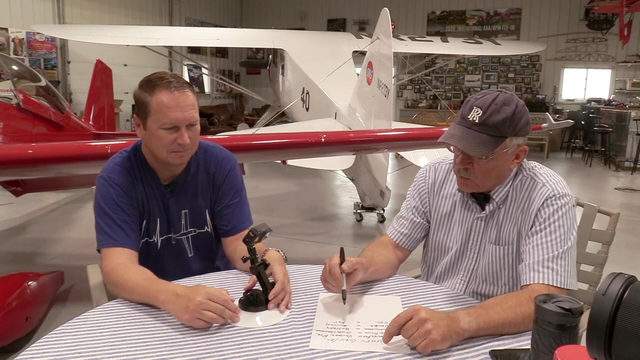 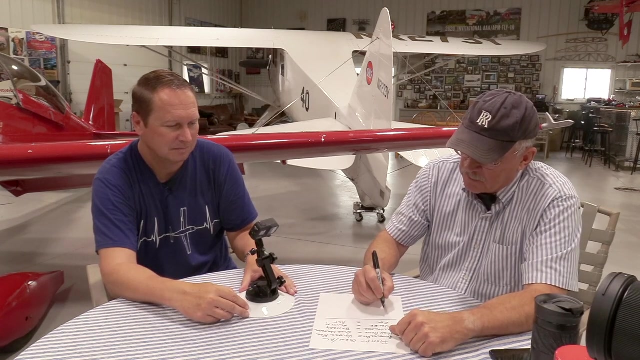 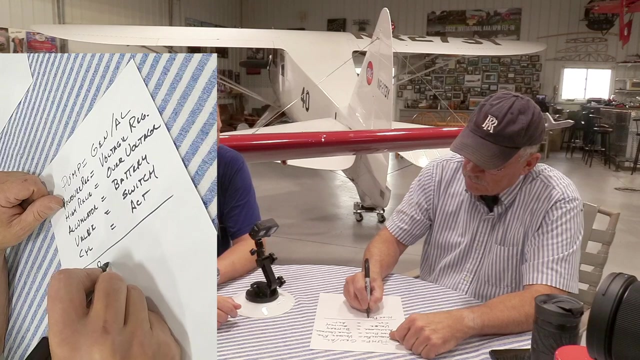 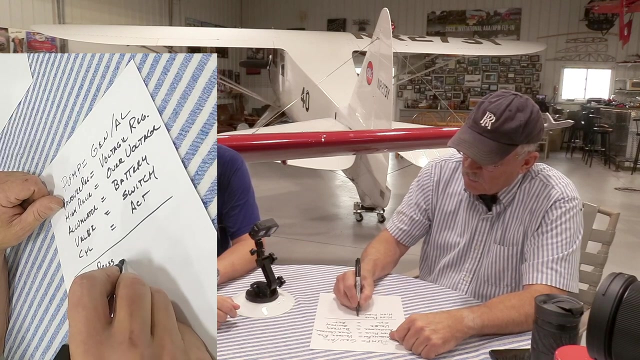 equals the battery, the valve can spell equals a switch, the cylinder equals a motor or an actuator, some electrical device, some electrical device that does work. so these would be the component comparisons and, as we look at diagnosing, if we have high pressure and high flow, we have high voltage, high. 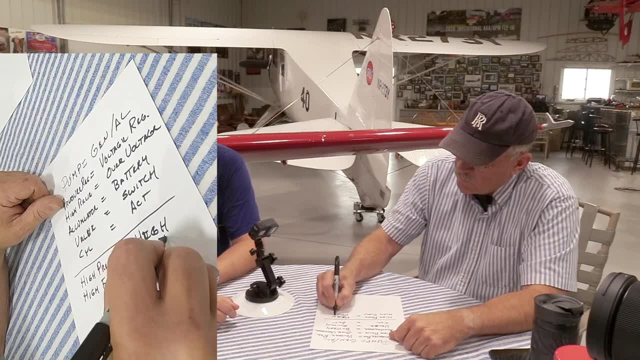 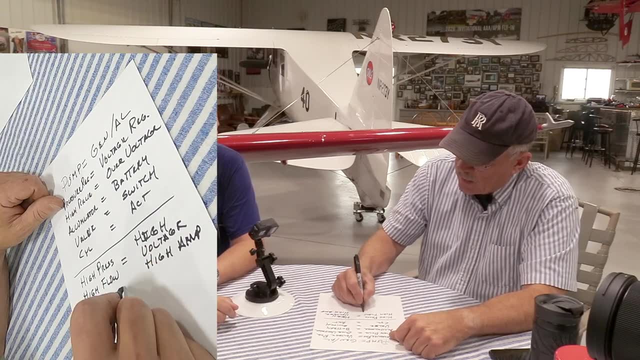 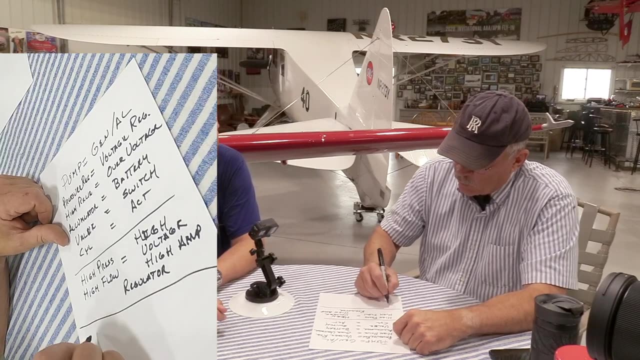 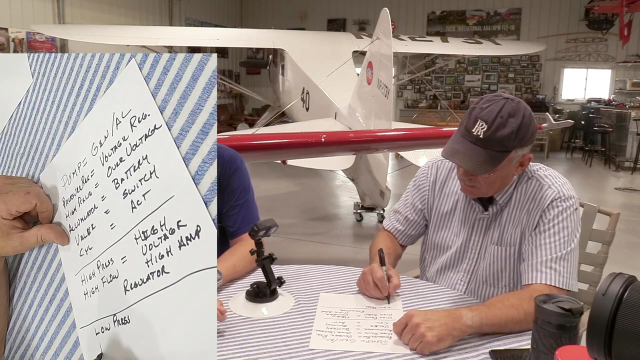 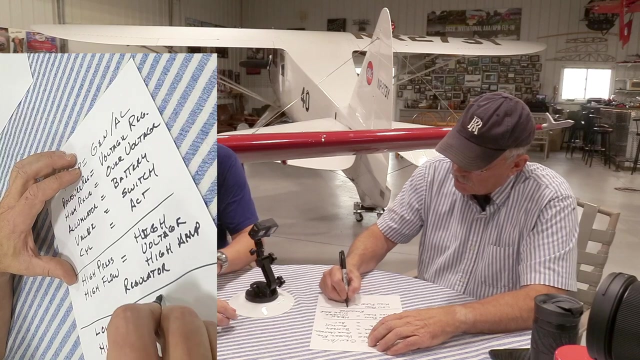 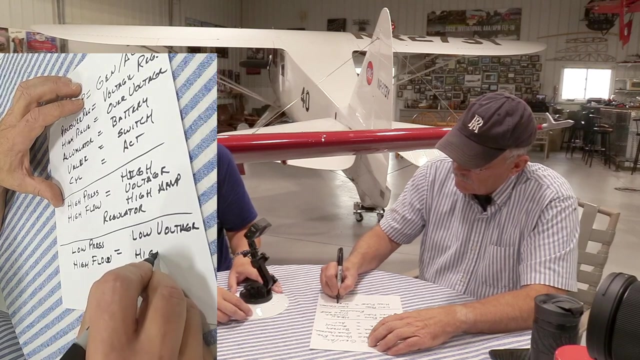 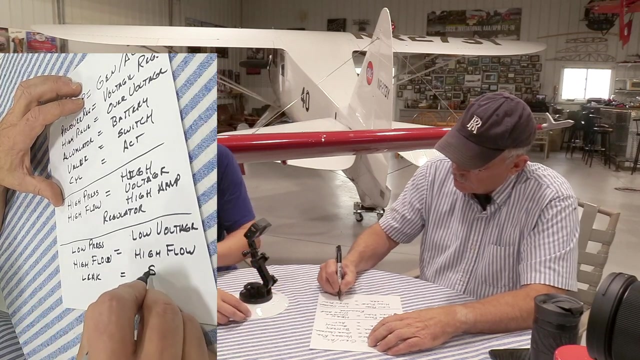 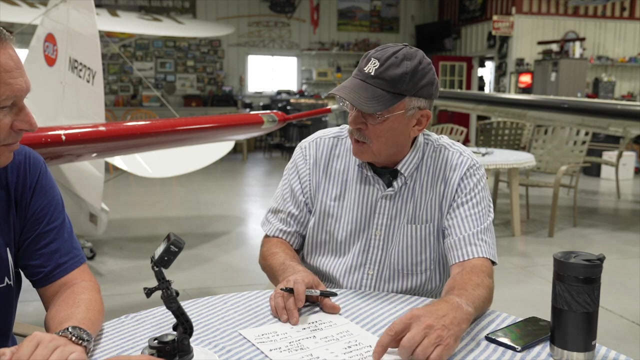 voltage and high amperage. that's got to be a regulator, almost has to be a regulator problem. and if we have low pressure and high flow, that equals low voltage and high flow and that equals a leak which equals a short. so if we think about electricity in the concept of hydraulics, I think it 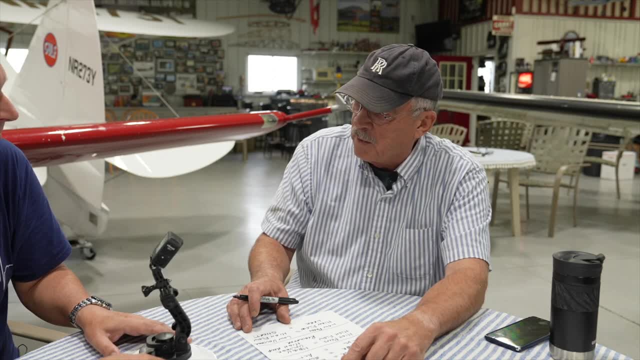 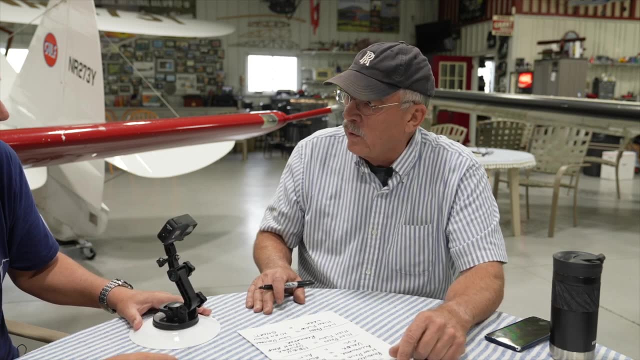 makes it a lot easier for a pilot to understand what's going on in their electrical system in their airplane and they can more accurately diagnose what's going on when they have a problem. yeah, the fluid is something we can see. we can feel its pressure on a hose. that's. 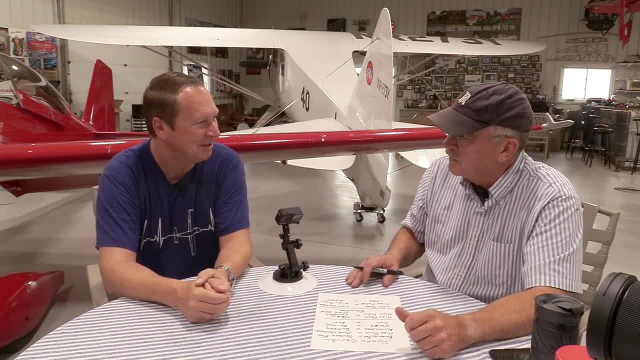 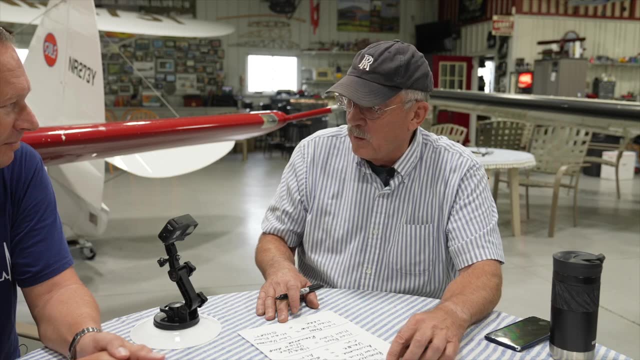 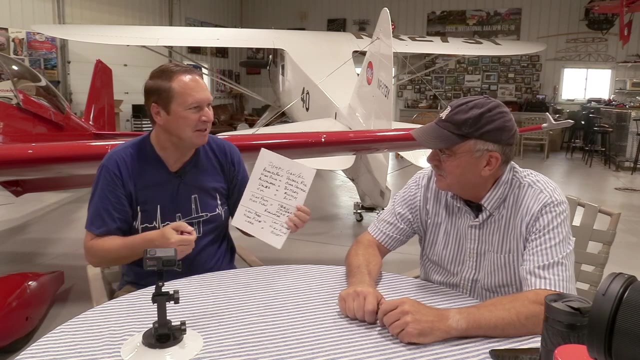 right. all of that makes more intuitive sense than thinking of electrons moving somewhere. so you know, I call this electrical electricity 101 for pilots. well, that's a really useful analogy here, and your pressure of the fluid and movement of a fluid is something we can feel, we can see. 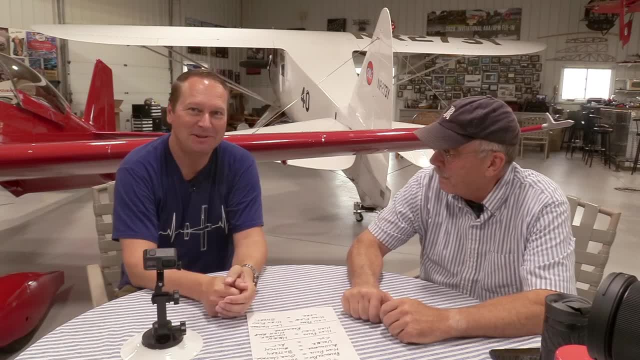 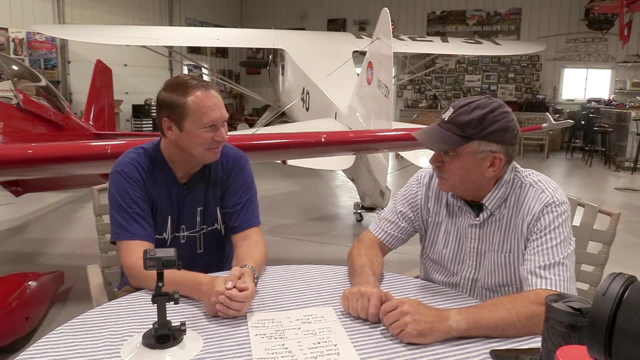 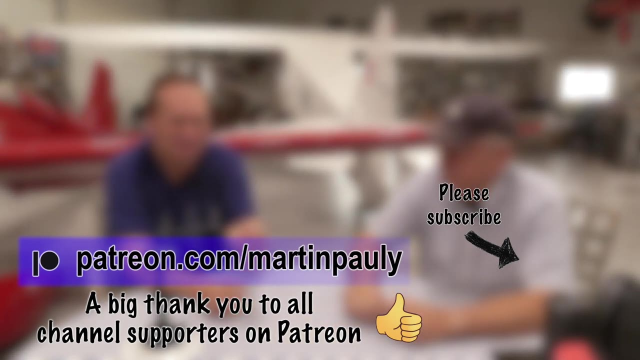 and that I hope will help understand how electricity works. thank you for explaining it and welcome. hopefully it'll be helpful. I think so. see you all in the next video. you. 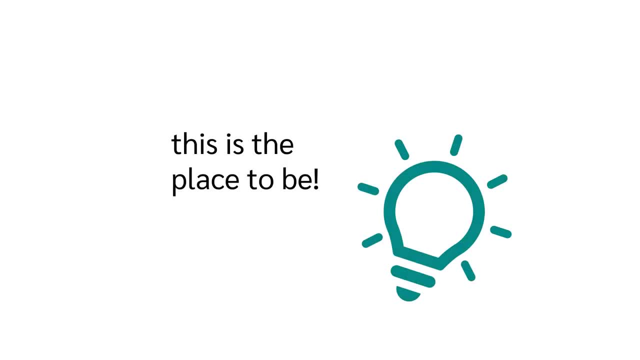 If you want to finally understand statistics, this is the place to be. After this video, you will know what statistics is, what descriptive statistics is and what inferential statistics is. So let's start with the first question: What is statistics? Statistics deals with the collection. 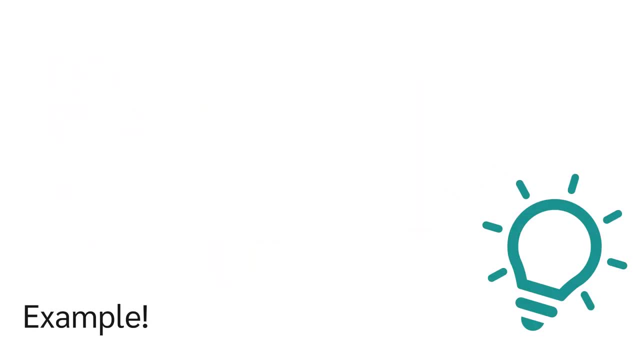 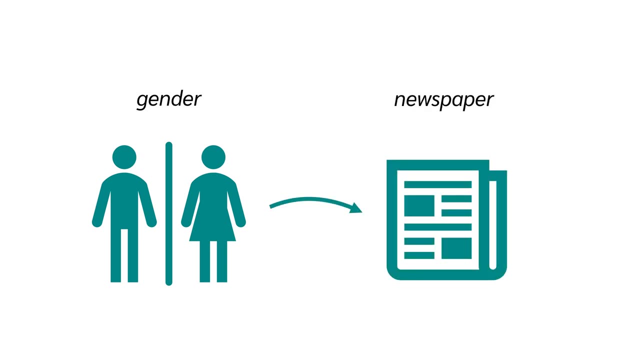 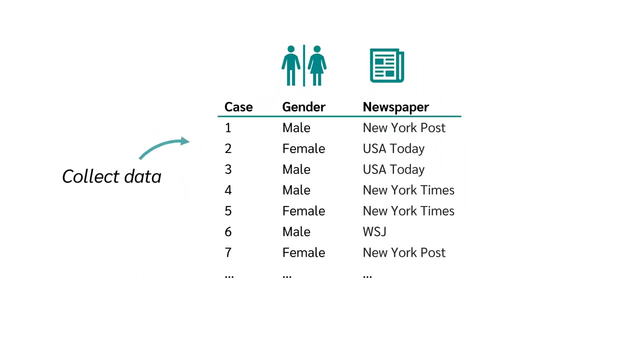 analysis and presentation of data. An example: We would like to investigate whether gender has an influence on the preferred newspaper, Then gender and newspaper are our so-called variables that we want to analyze In order to analyze whether gender has an influence on the. 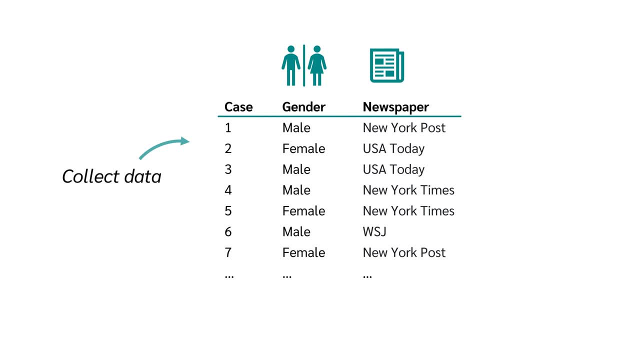 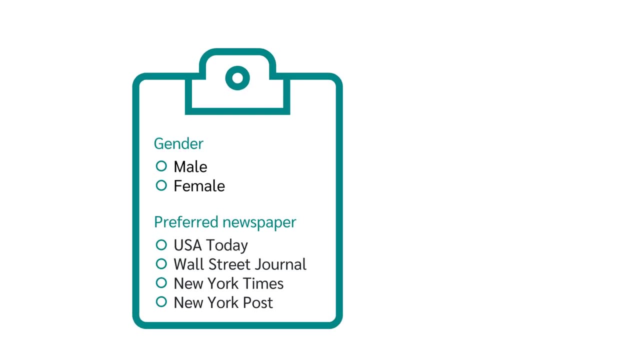 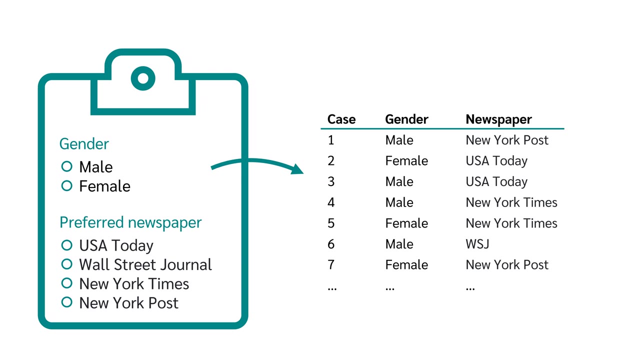 preferred newspaper. we first need to collect data. To do this, we create a questionnaire that asks about gender and preferred newspaper. We will then send out the survey and wait two weeks Afterwards we can display the receipts In this table. we have one column for each variable, One for gender and one for newspaper. 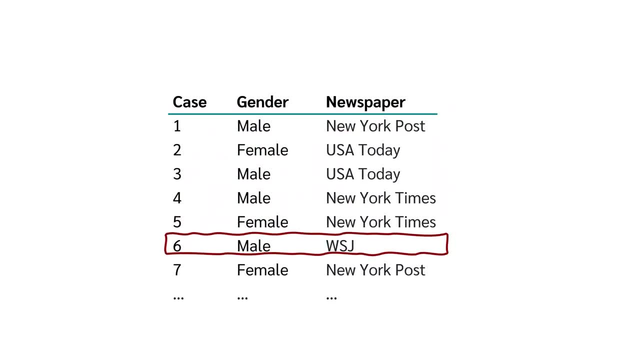 On the other hand, each row is the response of one surveyed person. The first respondent is male and stated New York Post, The second is female and stated USA Today, And so on and so forth. Of course, the data does not have to be from a survey. The data can also come from an. 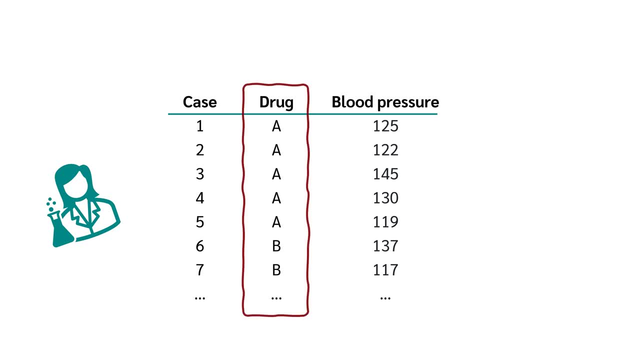 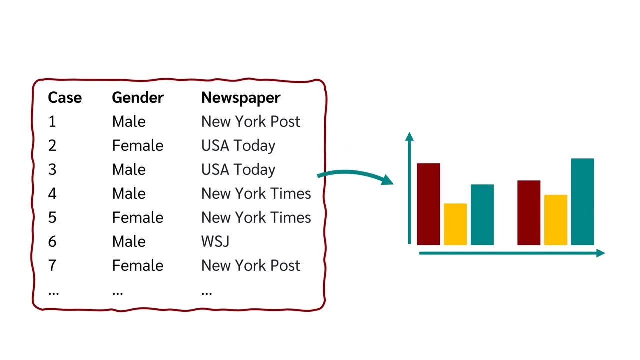 experimental survey. The data can also come from an experimental survey. The data can also come from example 2.. This is the document in which you, for example, want to study the effect of two drugs on blood pressure. Now the first step is done. We have collected data And we can start analyzing. 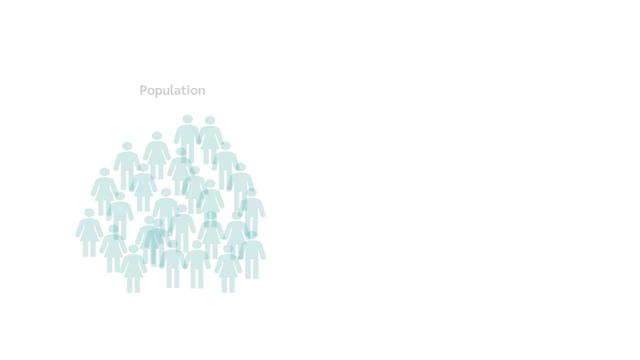 the data, But what do we actually want to analyze? We did not survey the entire population, but we took a sample. Now the big question is: do we just want to describe the sample data or do we want to make a statement about the whole population? If our aim is limited to the sample data?